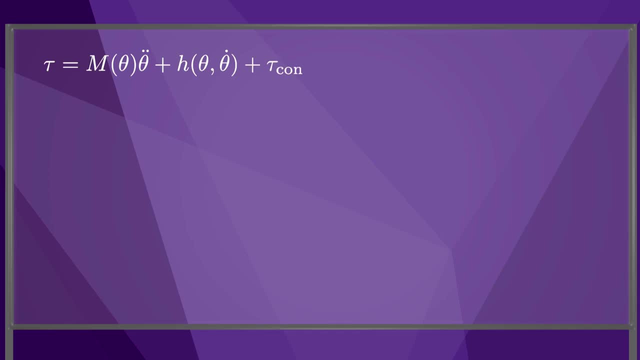 torques tau may include forces against the constraints tau-con. Thus the joint torques can be separated into components that move the robot and components that act against the constraints. Since constraints work less, the dot product of the torques against the constraints with 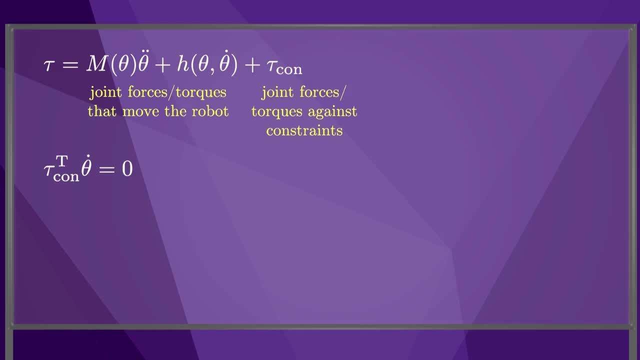 the joint velocities must be zero. We also know that the velocity constraints have the form a theta dot equals zero. so therefore the constraint torques must be a linear combination of the rows of a, where the k vector of coefficients lambda is called the vector of Lagrange multipliers. 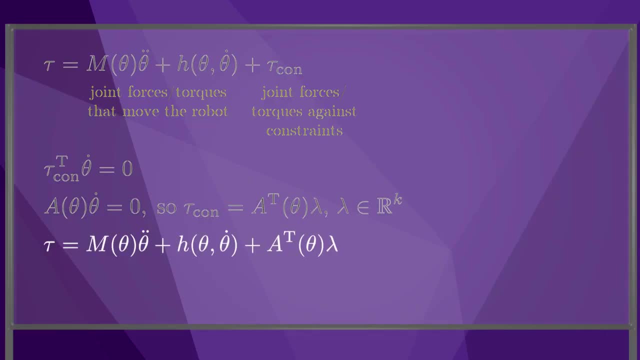 With this observation, we can rewrite our dynamics in this form: Since the velocity constraints must be satisfied at all times, we can re-write the dynamics in this form: Since the velocity constraints must be satisfied at all times, we can re-write the dynamics. 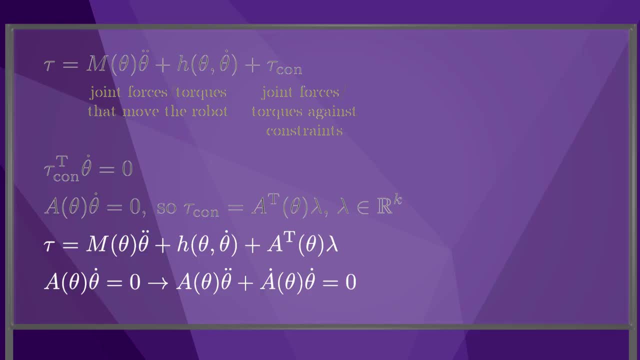 times they can be expressed as constraints on the acceleration. These are now n plus k equations in n plus k variables, the k-Lagrange multipliers in either n joint accelerations or n joint torques, depending on whether we are solving the constrained. 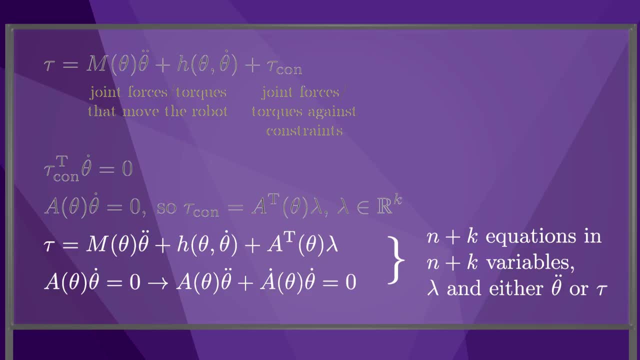 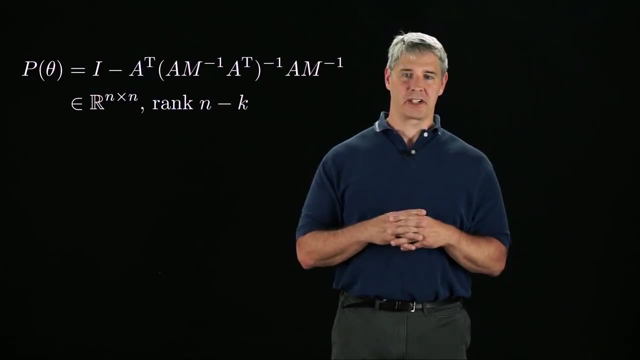 forward dynamics or the constrained inverse dynamics. Skipping the derivation which is given in the book. we can eliminate the k-Lagrange multipliers by defining an n-by-n projection matrix p of theta equal to the n-by-n identity matrix minus A transpose times the inverse of A- m inverse A transpose times A- m inverse. 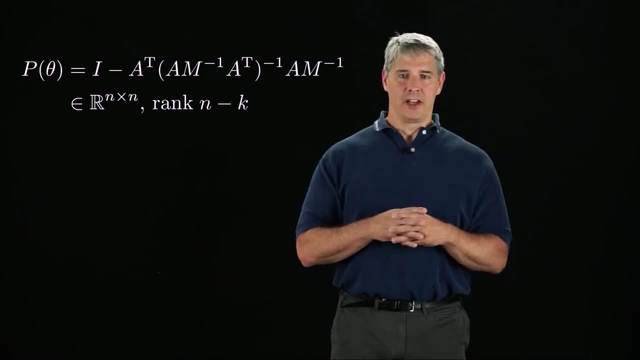 The rank of this n-by-n matrix is n minus k. Using this projection matrix, we can define the constrained inverse dynamics: p times tau equals p times m, theta double dot plus h. Since p is not invertible, we cannot pre-multiply. 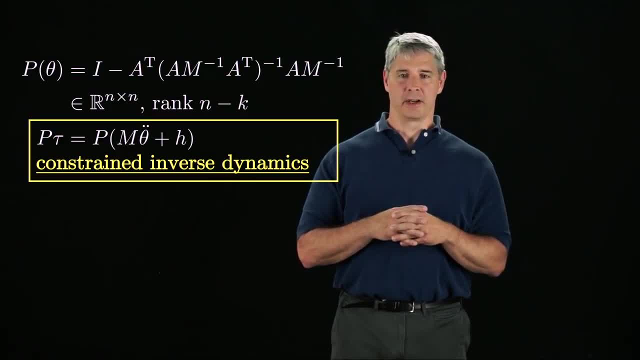 both sides by p inverse to get the unconstrained inverse dynamics. Instead, p projects the joint torques tau to the joint torques that move the robot, eliminating the joint torques against the constraints that cause no motion of the robot. To solve the inverse dynamics we plug in the joint positions, velocities and accelerations. 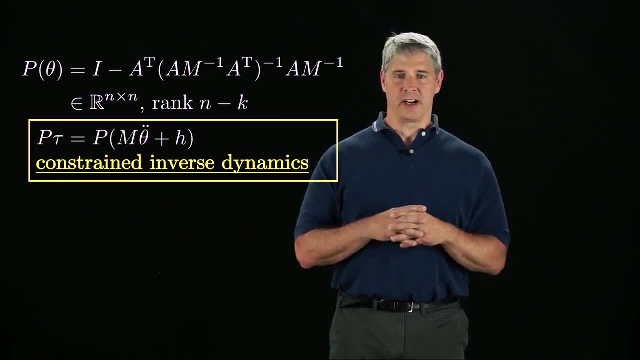 on the right-hand side to calculate the joint torques that create the desired joint accelerations. To this solution we can add any joint torques of the form A, transpose, lambda, which create forces against the constraints and do not affect the motion of the robot.